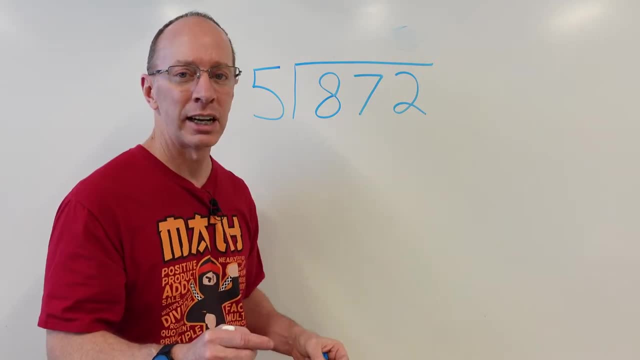 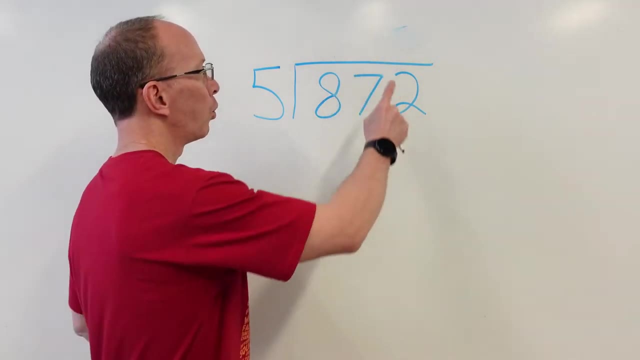 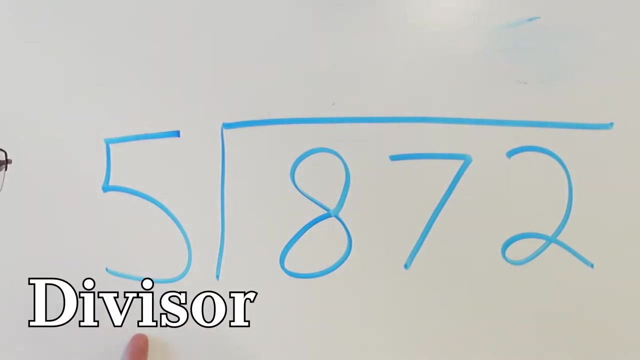 divide this number into five equal groups. That's why you're a math ninja. Five equal groups, All right. And then we put our answer, our question. All right, Remember, this is the dividend, the divisor. answer of the quotient. All right, Ready. 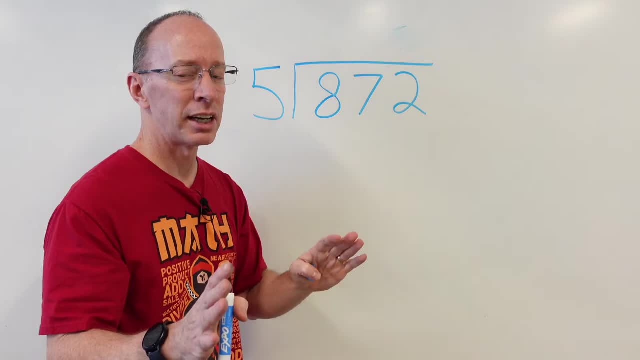 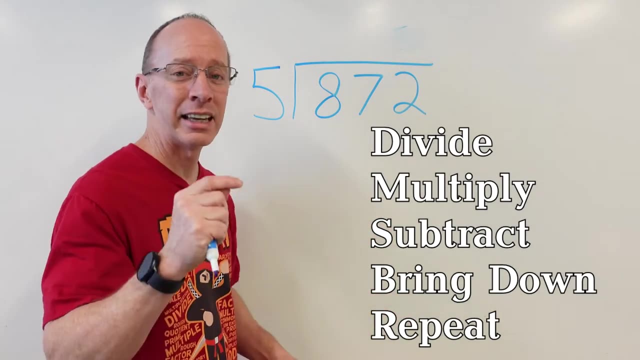 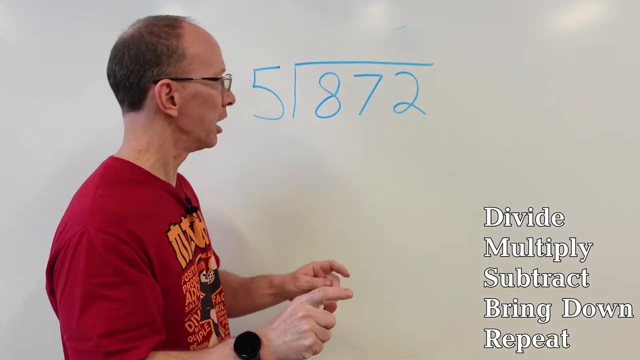 to get started Now, before we get started, there are some steps. We have to first divide, multiply, subtract, bring it down and then repeat. if we have to keep on going, All right, But I'll work you through these steps, All right? All right, Hang on there, Let's get started. Yeah, All right. 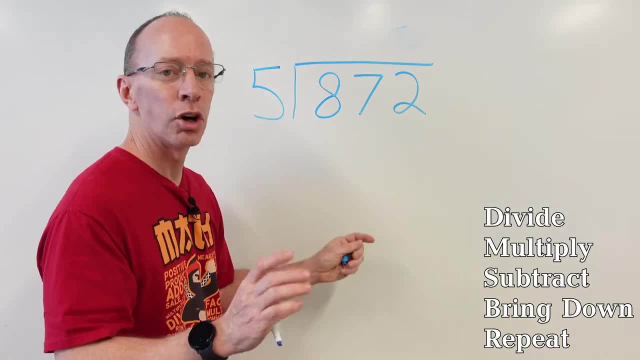 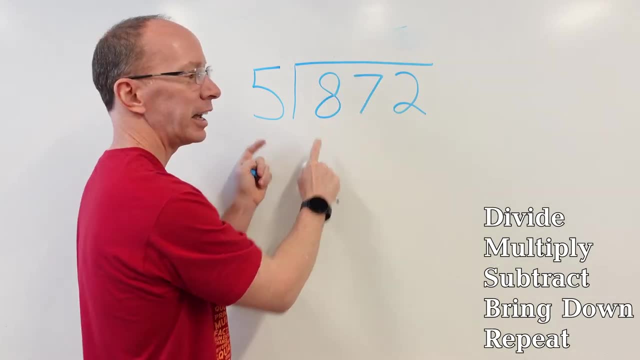 First of all, we have 872.. Don't get worried, That's a big number. Ignore those numbers. First of all, five. Can I put five into eight? Yes, Yes, you can. How many times can I put five into eight? Five times one is. 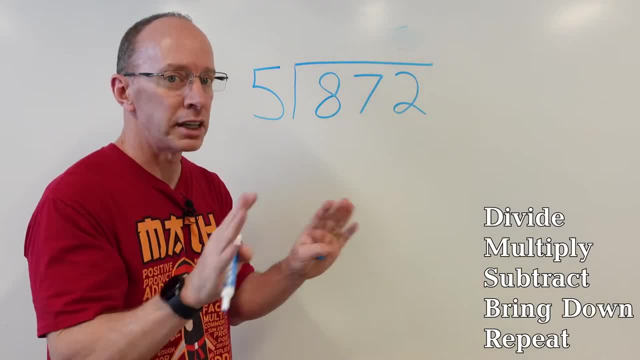 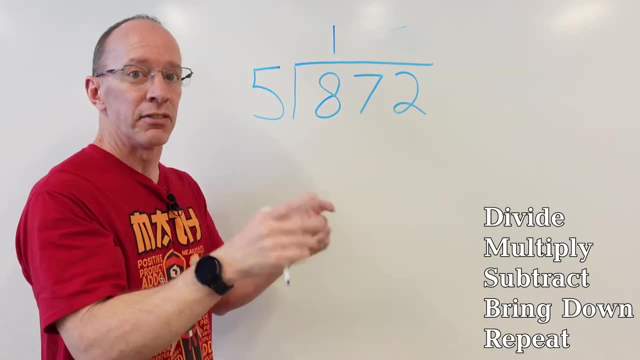 five. Five times two is ten. No, don't go to ten, That's over it, Just once. Five times one, All right, Five times Now. we did the first step, That was dividing. Now I have to multiply One times. 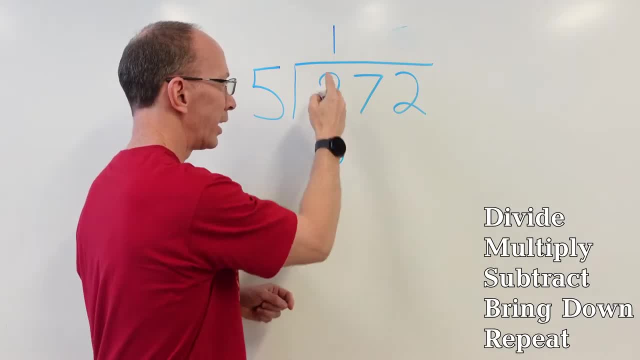 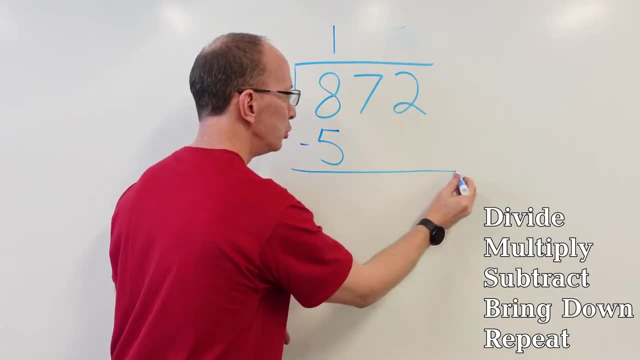 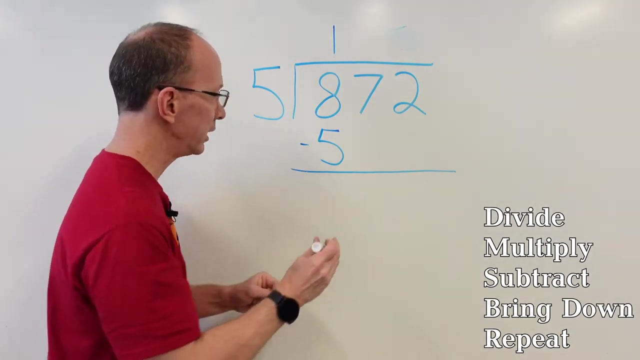 five is five. Okay, Put the five right there. Okay, You're dealing with that number, right there. Okay, Put a little line there, Right there, All right, Make math fun. Yeah Now. eight minus five, What is it? Three? Uno dos tres, All right, Can I put five into three? Always check that, Can I? 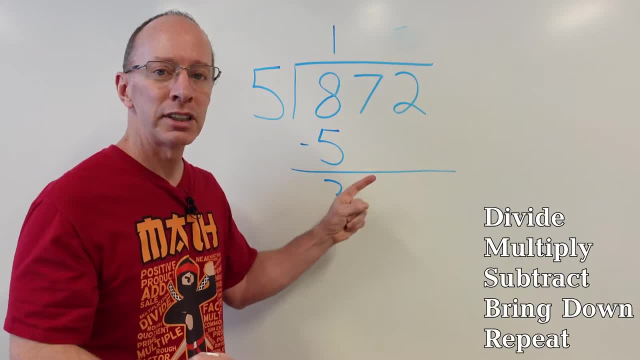 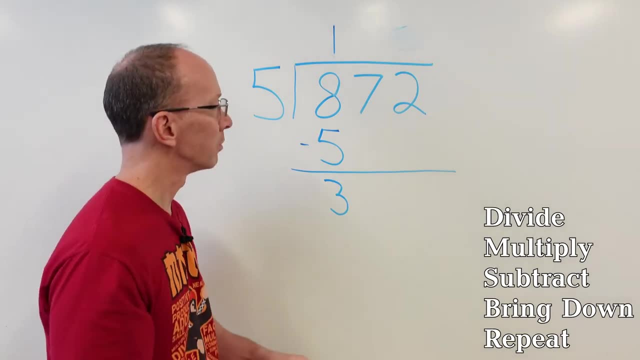 put five into three. No, you can't. Now I move to the next number. All right, Remember what we did. We divided, Multiplied Subtract. Bring it down, Bring it down, You drop it down. Boom, Right here. 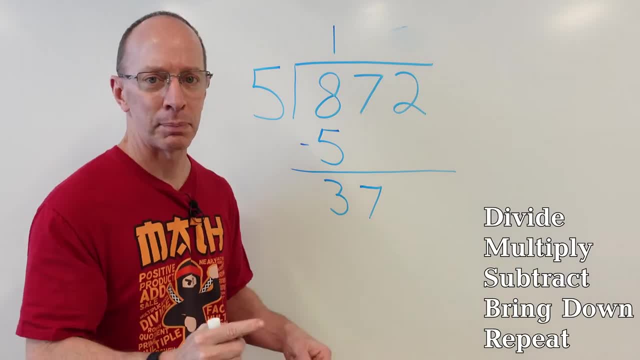 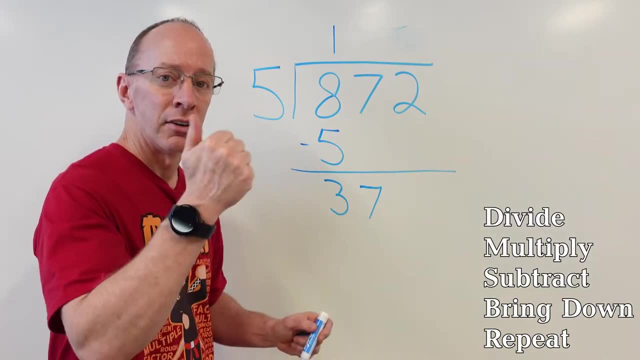 Put that seven right here. Drop it down, All right. You can bring it down or drop it down. I like the sound of it. Drop it down, All right. Now we got to put five into 37. Can we do it? Let me see 5,. 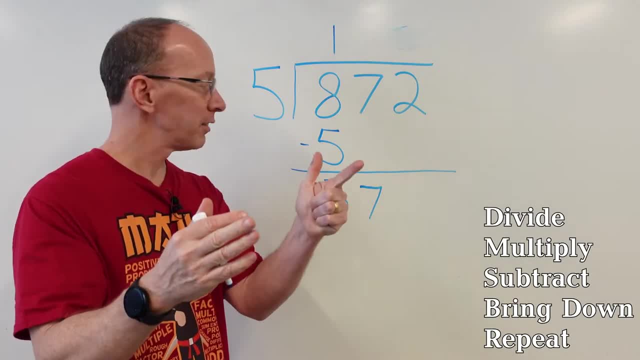 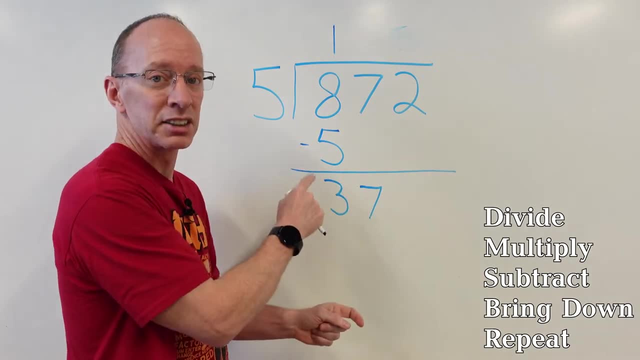 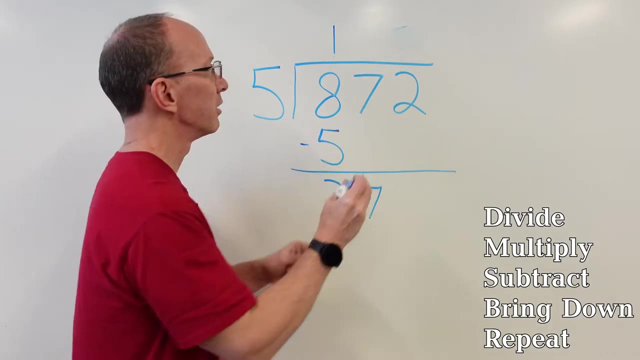 10,, 15,, 20,, 25,, 30,, 35,, 40.. Forty Too high, All right, I'm getting my fingers all mixed up. Five times seven is 35. Let's stick with seven. I think that's a good number, All right, Put the seven. 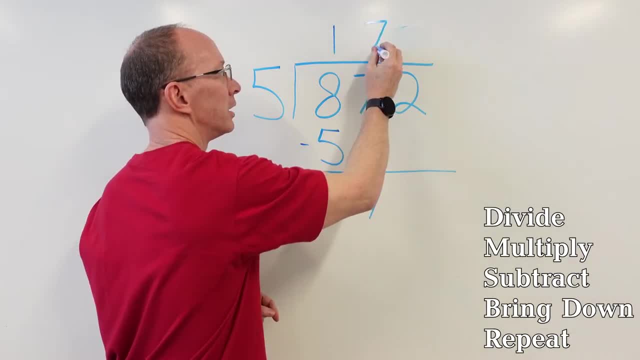 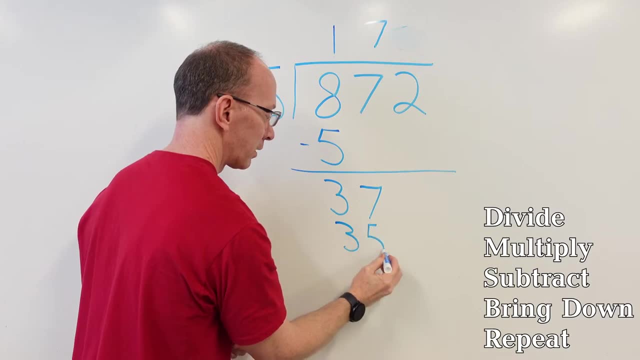 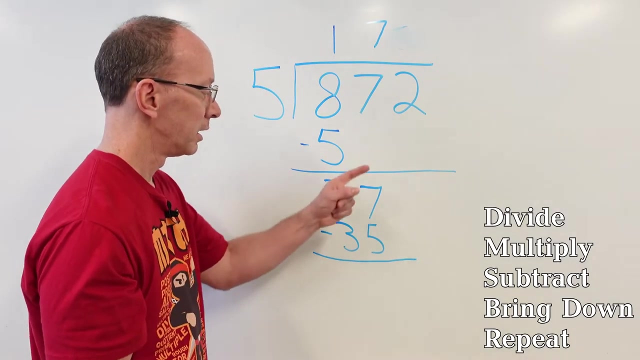 right up here. Okay, Right up here. We divided. Now we multiply Seven times five is 35. Okay, What's the next step? Subtraction. Here we go. Subtract it, All right, Always subtract the ones first. Seven minus five, Five, six, seven, All right, Two. 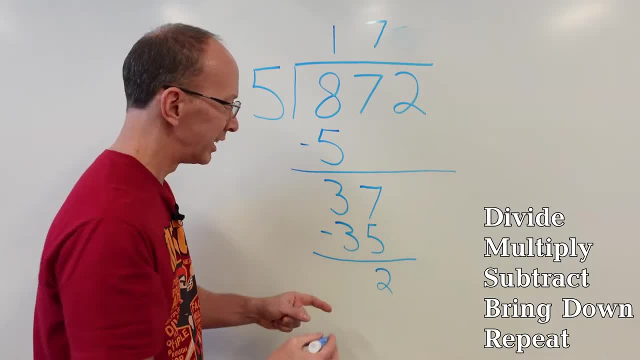 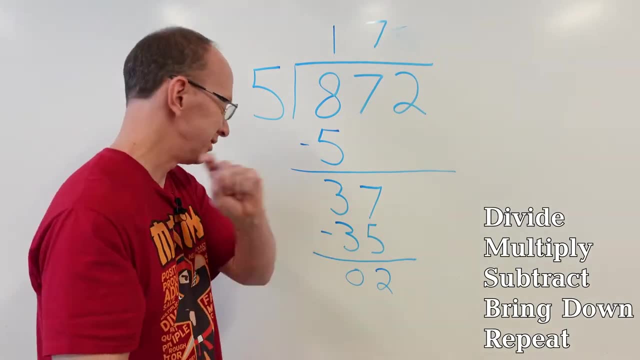 Three minus three Zip Zero. Don't put that zero there. If you put the zero there, you can, but you don't say 37 minus 35 is zero too. No, Just ignore it. It's nothing, Okay. Two: 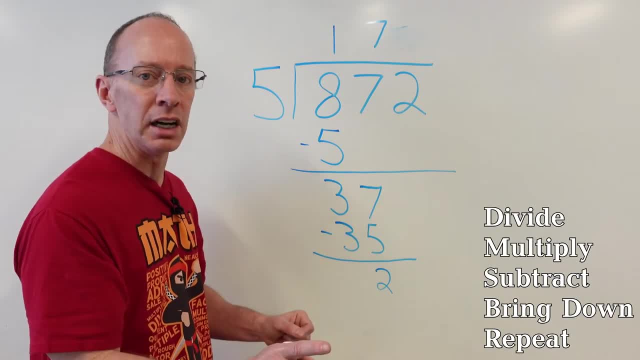 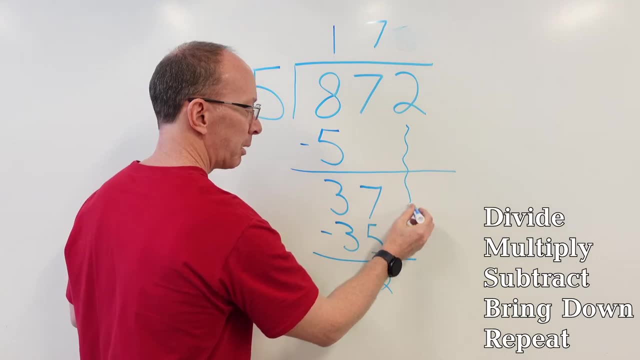 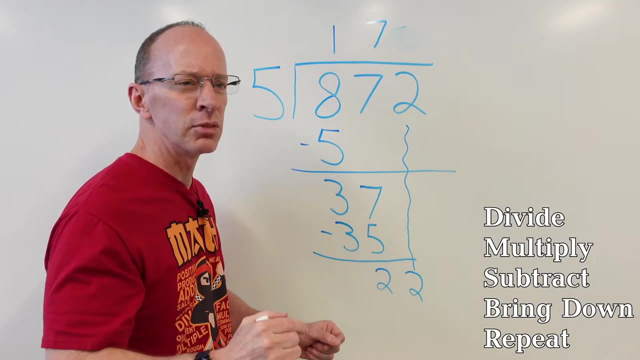 All right. Next step: Repeat: Yeah, All right, Drop it down, Drop it down. We bring that two down. All right, A little beatboxing for you. All right, The teacher's probably over there saying: get on with the lesson, Come on, All right, All right. 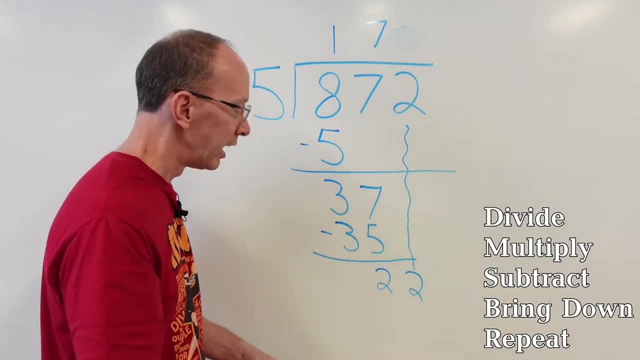 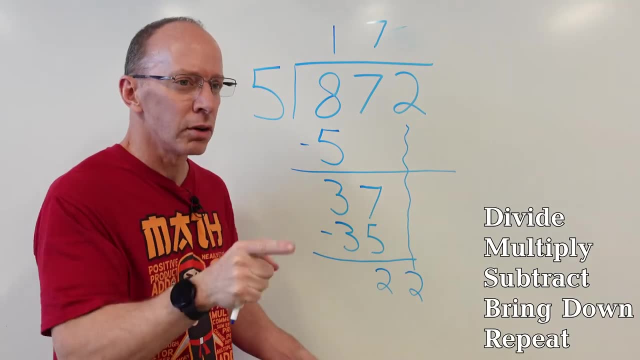 All right, Okay, Now got to do it again: Divide. How many times can I put my five into 22? 5, 10,, 15,, 20,, 25.. No, no, no, no. Five times four is 20.. Five times five is 25.. Too high, Just do five. 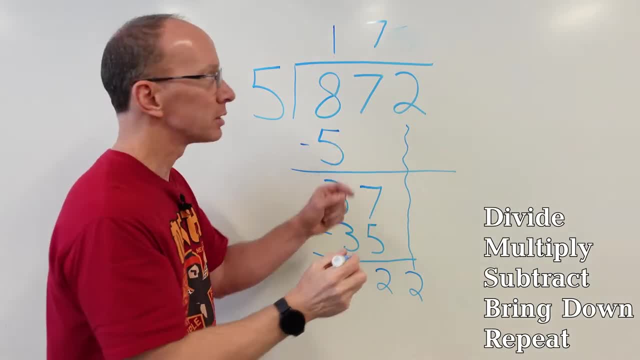 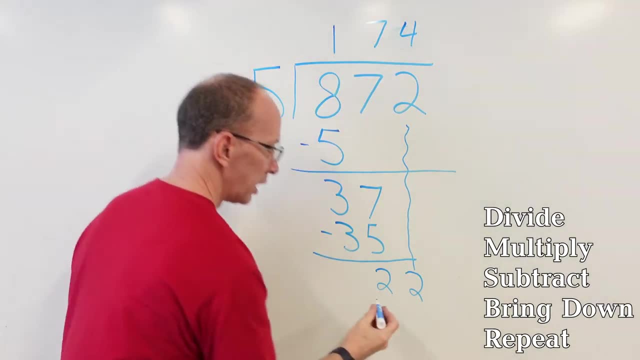 times four, Can we do it? Yeah, Don't forget to put the four up here. Four, All right, Now we multiply. The next step: multiply Four times five is 20.. Right there, Next step: subtract. You guys are getting so good, That's. 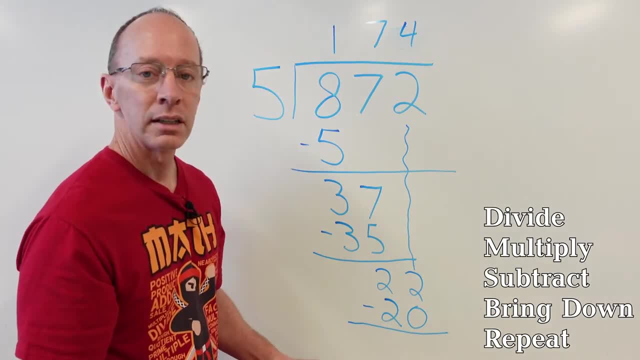 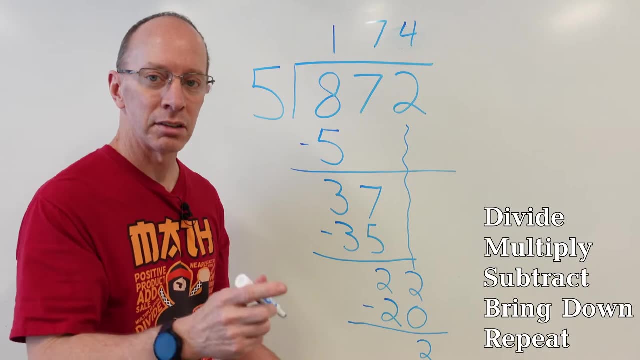 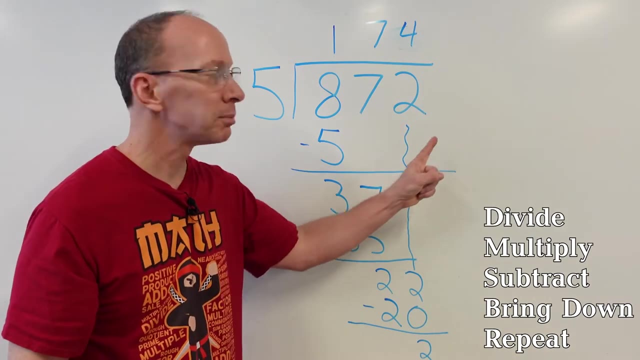 why you're a math ninja just like me. All right, Let's subtract it: Two minus zero Two. Two minus two, Zip Zero, Nothing, Okay. Next step: You brain it down. All right, Drop it down. There's no number to drop it down. That's it, We're done, We're finished. We have this two here. 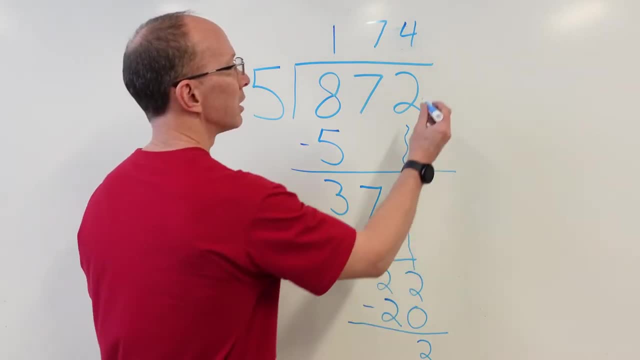 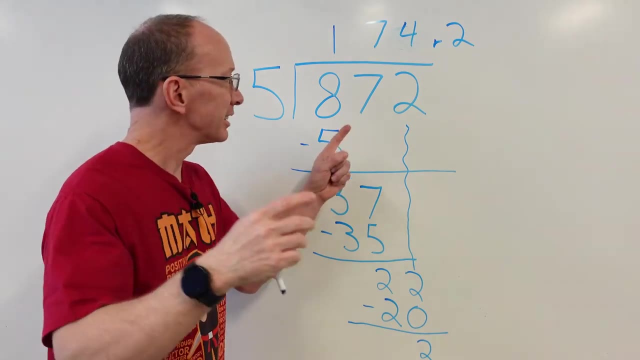 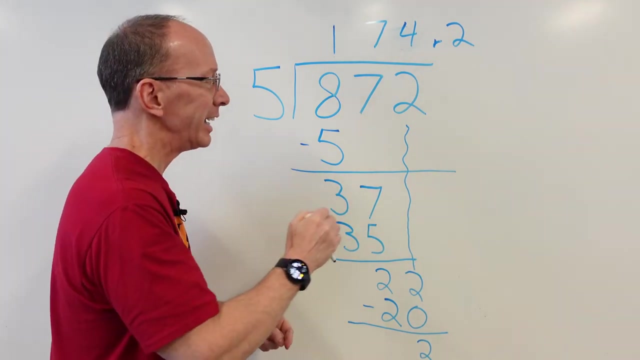 That is a remainder, two, All right. So we put a little R right here for the remainder and we put a two. So when we are dividing this 872, those 872 pieces of candy, we're giving them to five groups, All right, In each of those groups- here is each of those groups- We have one group. 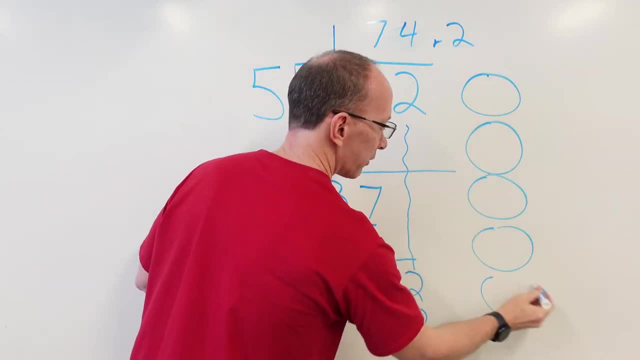 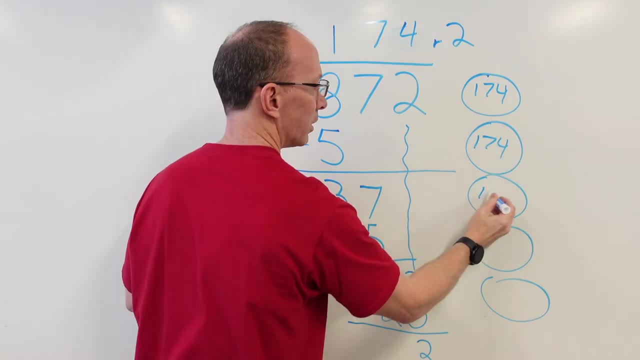 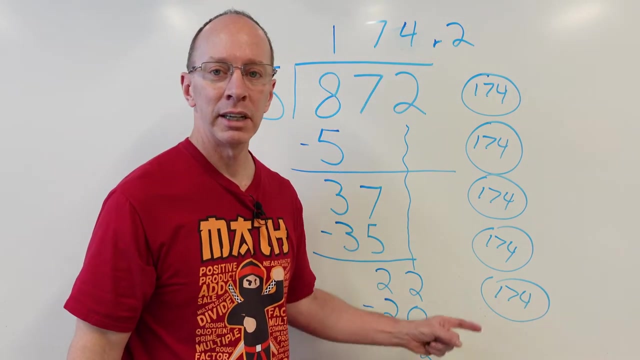 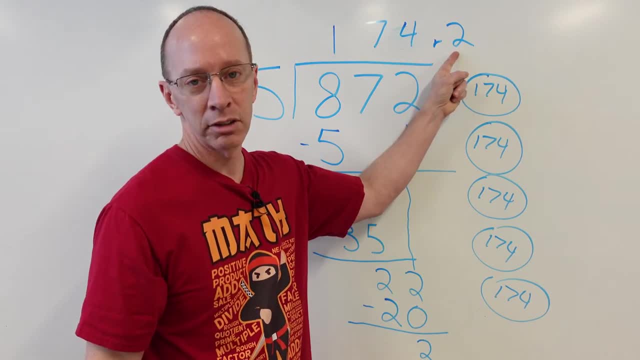 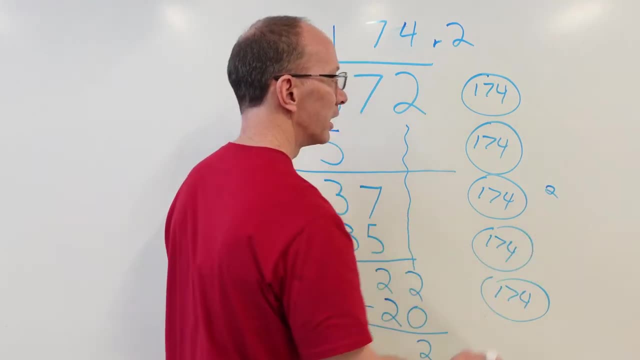 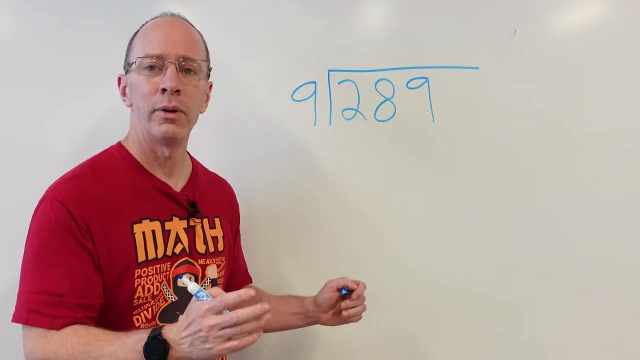 candy, And now I got a remainder of two and you can give those two pieces of candy to me because that's just enough. All right, You got two pieces left over. All right, There it is You ready to do another one? One more? Yeah, Let's do it. Yeah, Boom Okay, We got the number 289.. 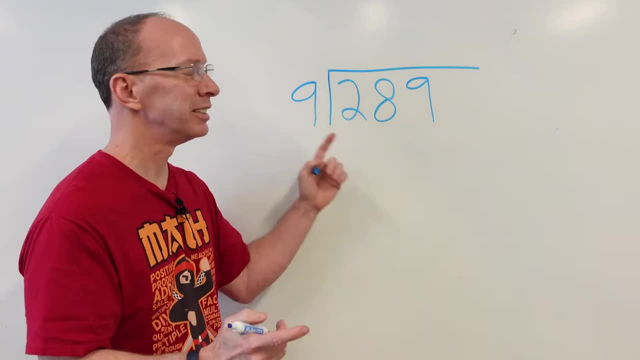 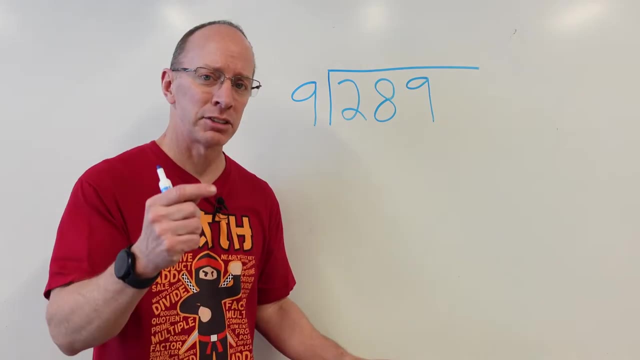 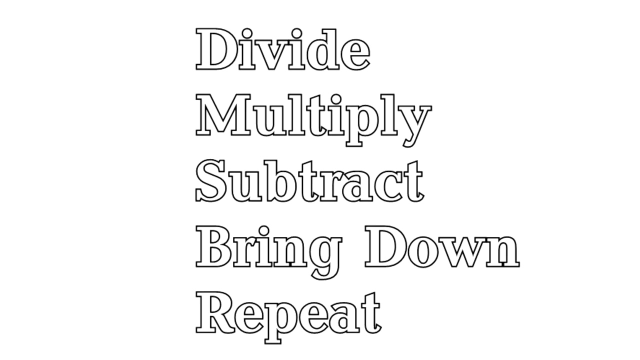 Divided by nine, That means we're going to put it into nine groups. We got 289 pieces of candy. I don't know where you guys are getting all these candy. Maybe we're out trick-or-treating last year And you got to give it to nine people. Okay, Let's do it. We got different steps. We divide. 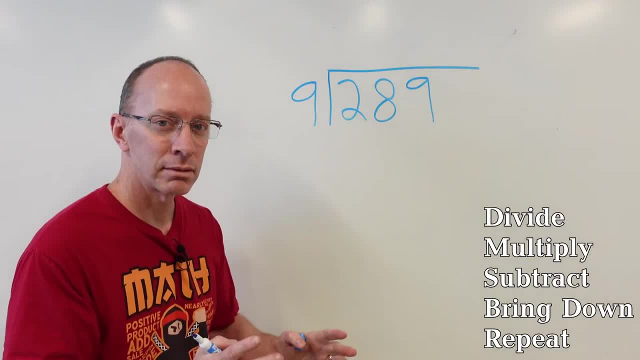 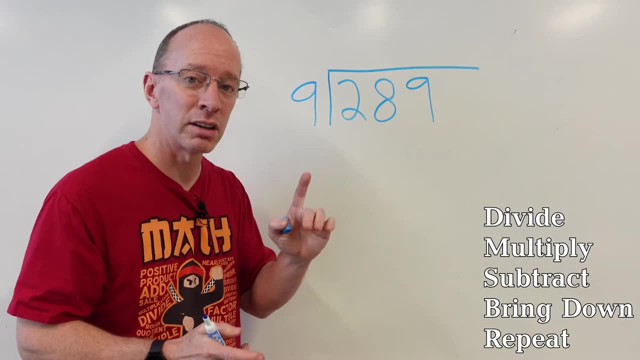 multiply subtract, bring it down and repeat. Okay, Let's do this one just a little bit kind of faster for you. Okay, Now, if you want to, you can pause the video and try this one and then check your answer. So go ahead and pause the video. 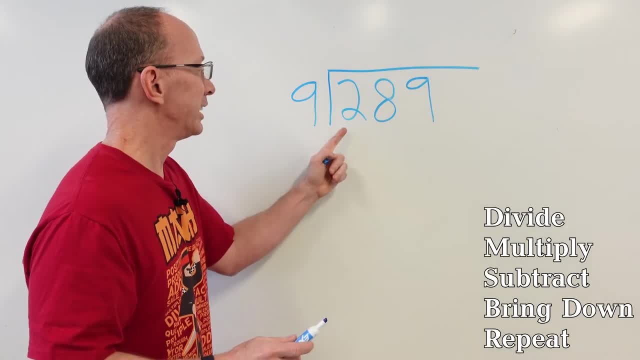 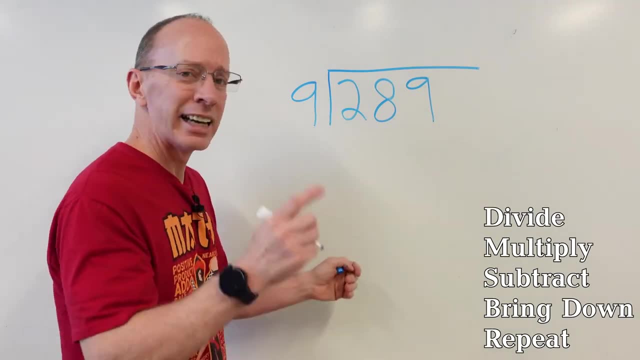 Okay, Let's do it. Yeah, Can I put nine into two? Let me see here. No, You can try to put that nine in. You can't do it. You just can't do it. Nine times one is nine. You got to go over to the next. 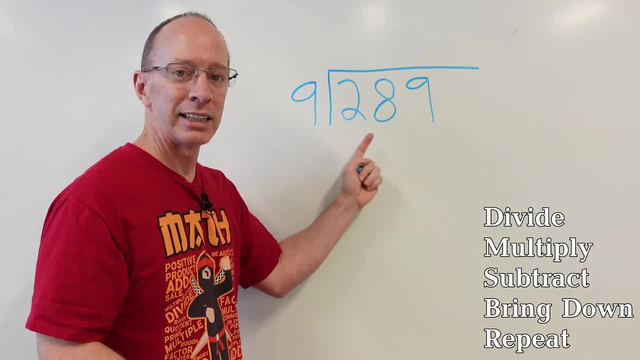 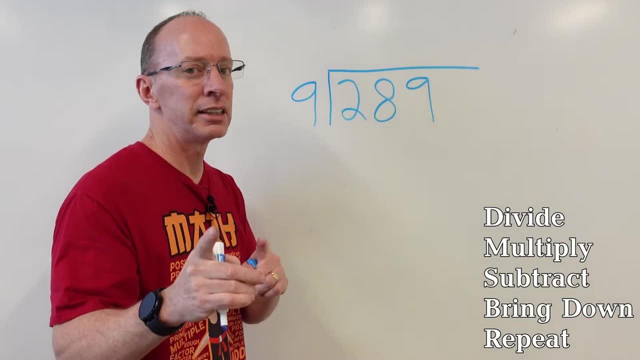 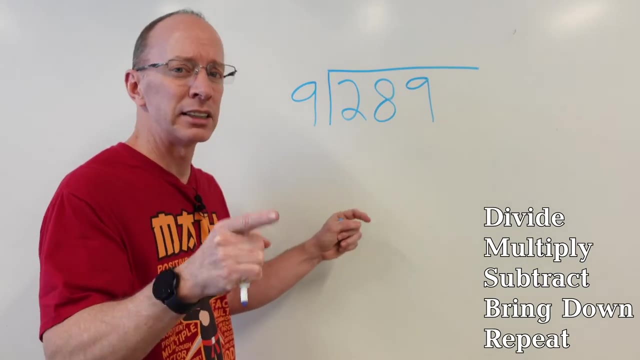 number here. Okay, How many times can I put nine into 28?? Nine times one is nine. Nine times two is nine. Nine times three is 27.. You got to know your multiplication facts, All right, If you don't study them, Okay, All right, I can do it three times. Nine times three is 27.. Put the three. 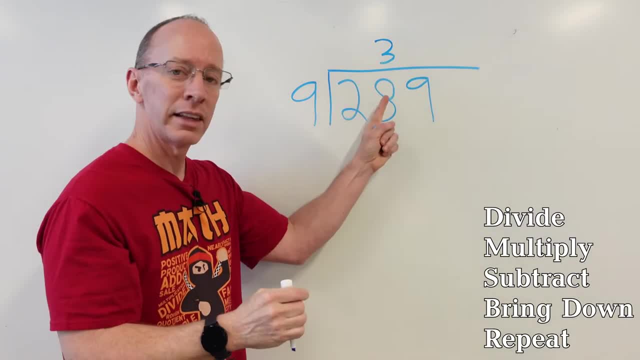 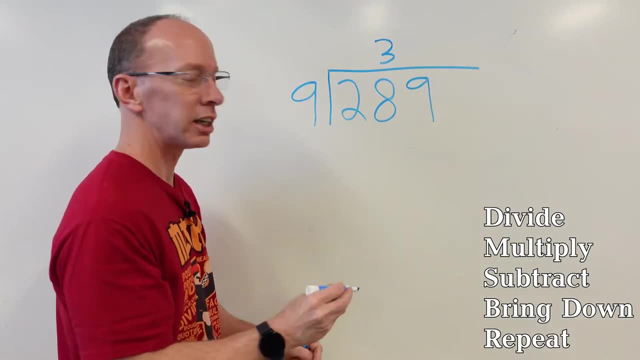 above here, Not over there. No, Right there, Because you're dealing with the 28. now, Okay, Next step: Multiply Three times nine is 27.. All right, 27.. All right, Put the line here. What's? 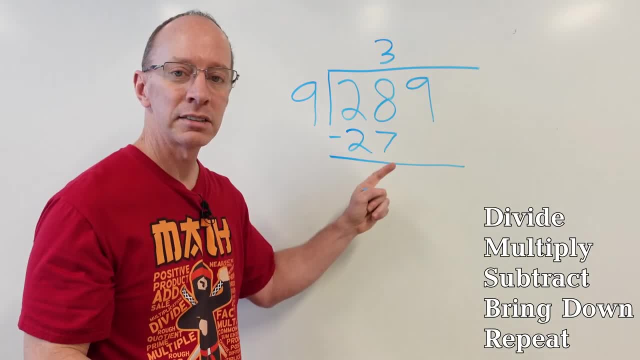 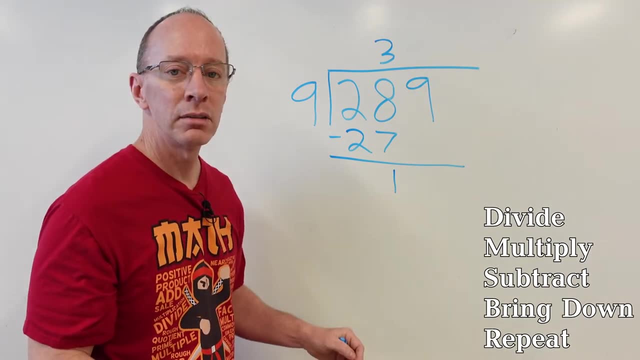 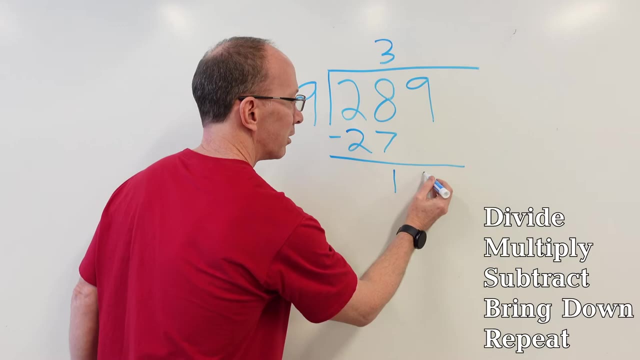 the next step: Subtract: Yeah Minus seven. One. Two minus two. No, Just zero, Just zero, Just zero. Now, what do you do? Bring it down, Bring it down. Bring that next number down: Yeah, Bring that down, Right here, Right. 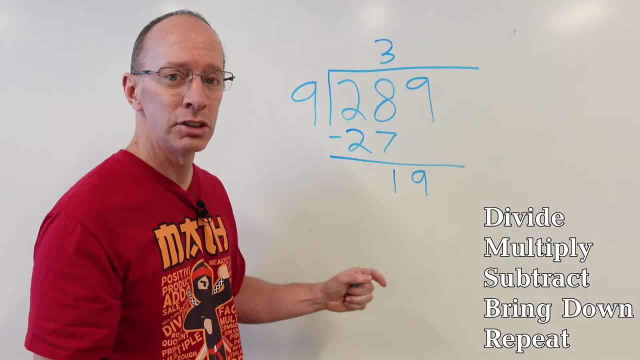 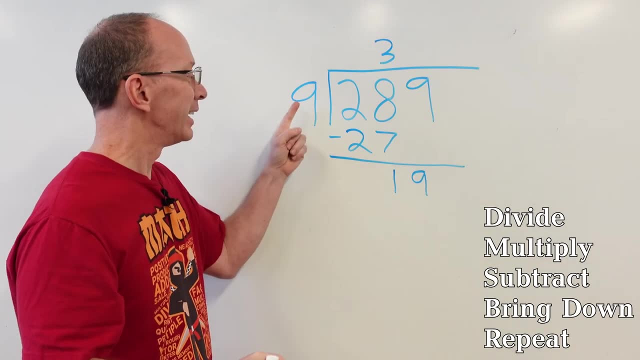 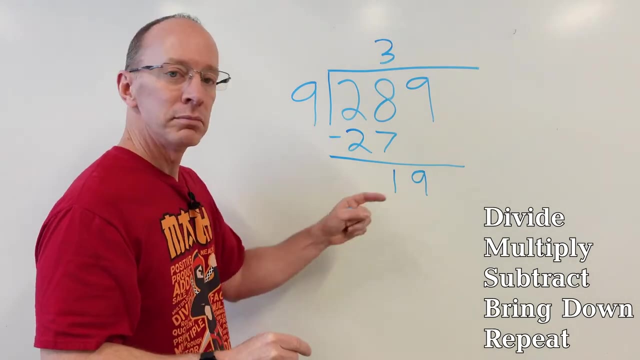 here, Yeah, 19.. Now we got to start over again. All right, We got to start over again. Repeat, Repeat, All right. How many times can I put nine into 19?? Nine Nine times two is 18.. Yeah, Two times, Two times. Put that two right above there Two. 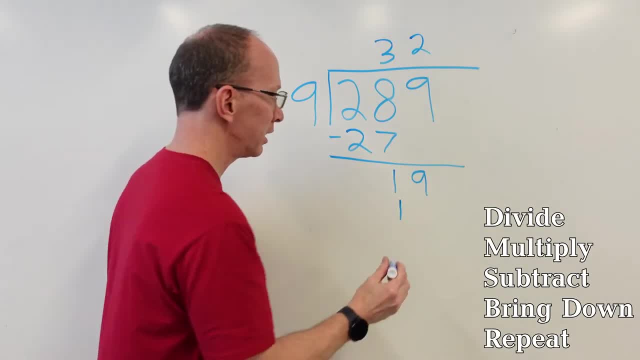 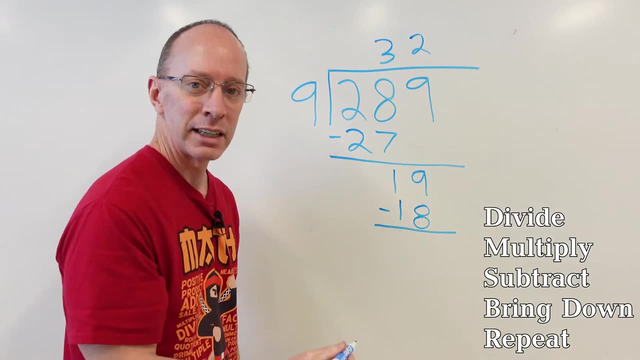 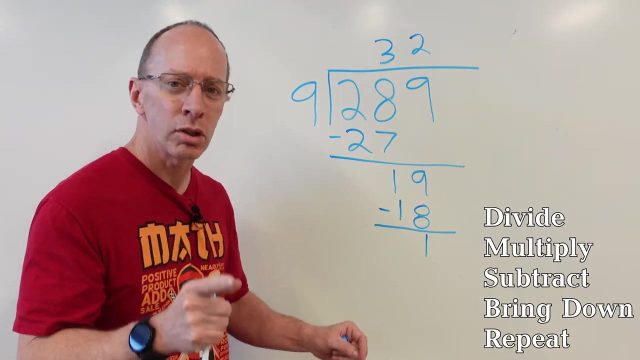 times nine is And we're multiplying. That's the next step, 18.. Now we subtract: All righty Nine minus eight, One Uno, All right, I love that song by Ricky Martin: Un dos tres. Okay, That's all I know of the song, But anyway, Uno One. 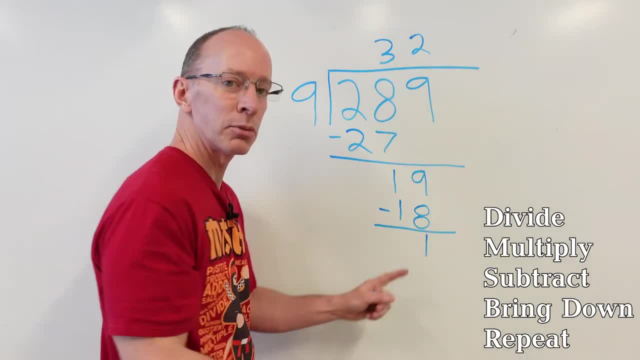 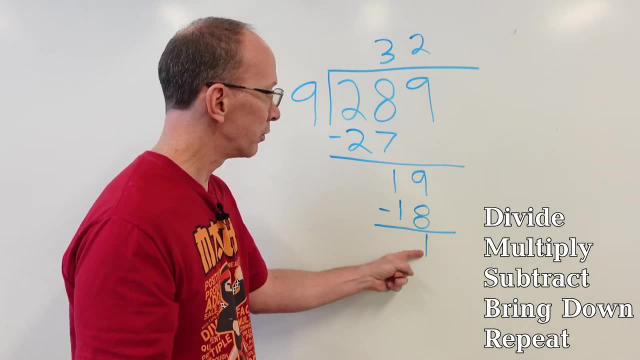 All right, That's our remainder. You can't put nine into the one anymore. If that remainder was bigger than nine, you got to keep on subtracting. But it's nine. That's the remainder. Throw it up here with an r. 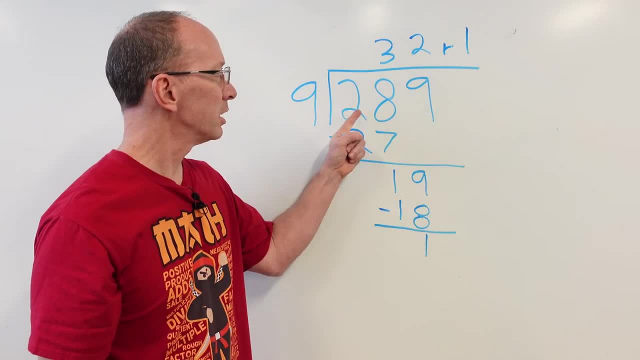 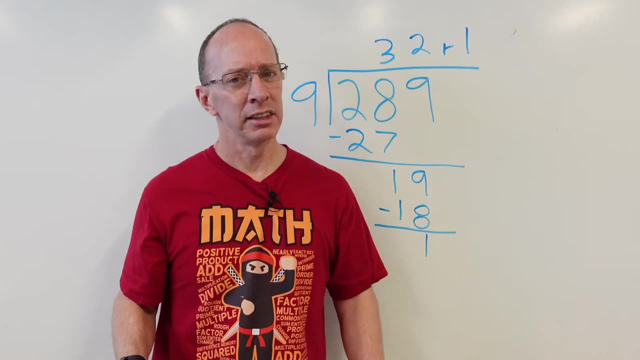 Remainder one. What is our problem? 289 divided by nine equals 32.. Remainder one: Yeah, you did it, my math ninja pro friends. Yeah You, yeah, you did it. yeah, all right, hey, make sure you check out my other videos on here. got a lot of. 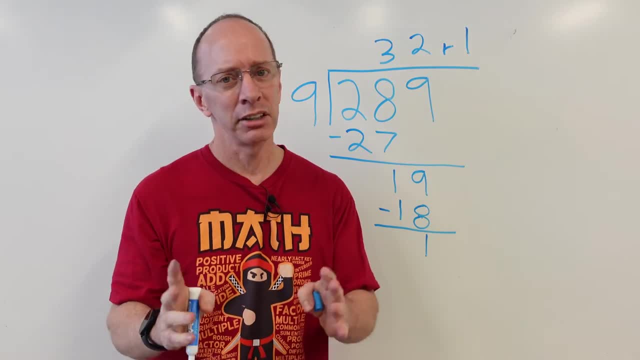 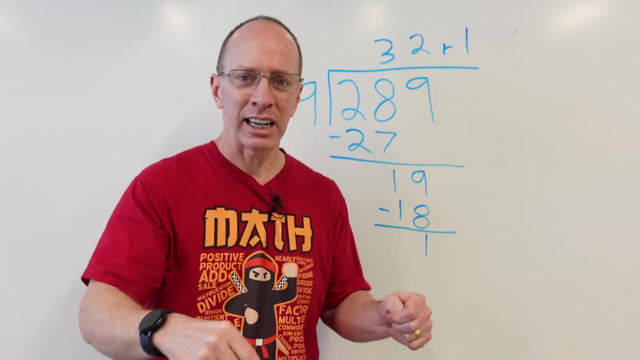 cool videos, even drawing videos, and please subscribe. tell your friends, call them up, yeah, tick, tock them, facebook them. whatever you have to do, get subscribed subscriptions on here. i'd really appreciate it and make sure you have a fun day. yeah, that's what i wanted to say. have a. fun day, adios. 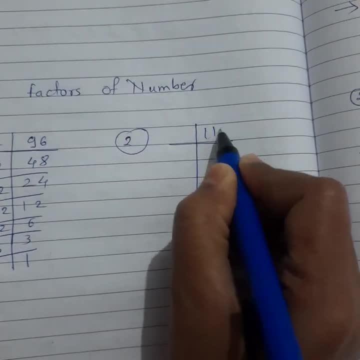 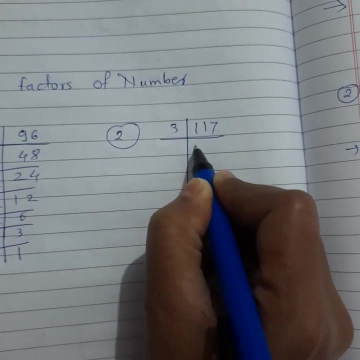 Factors of odd number, that is 117.. 7 plus 1,, 8 plus 1, 9,- 9 is in 3's table. 3- 3's are 9, 3- 9's are 27,. 3- 1's are 3, 3- 3's are 9, 13- 1's are 13.. 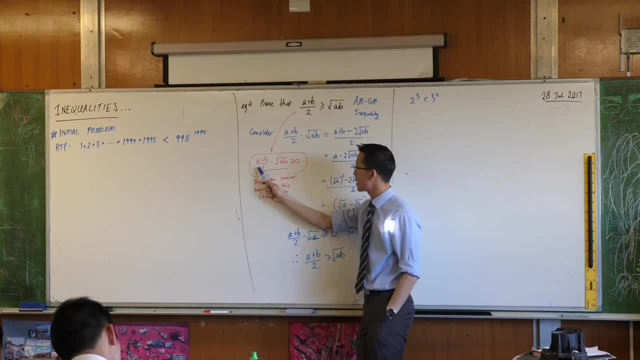 The question was: you know this thing here, the sort of overall mental strategy I was suggesting, which was move everything over to one side. You may have noticed, I talked it through with you, but I was very conscious of not writing it down right. I didn't actually say da-da-da-da-da-da.